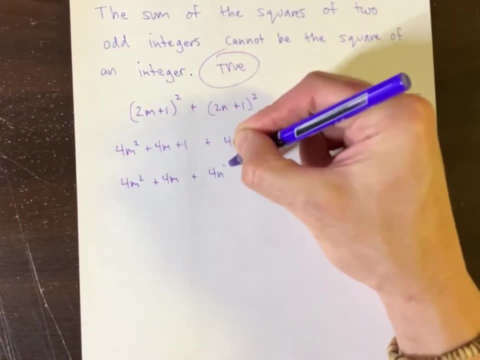 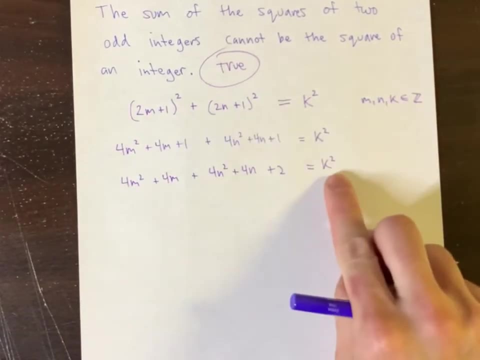 plus 4m plus 4n, squared plus 4n. I'm going to combine the 1 and 1 to give us a 2.. I'll leave the k squared alone. Now, what I want to do from here is: 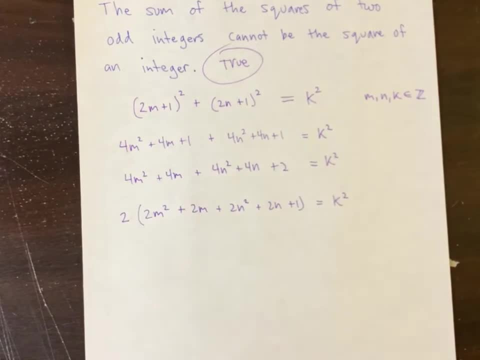 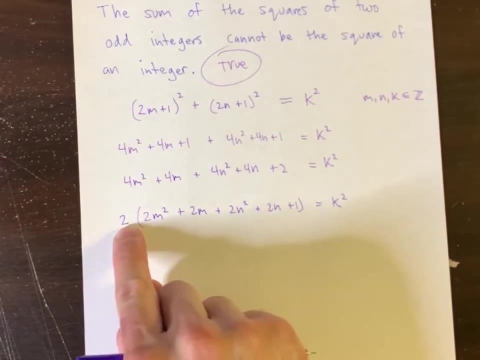 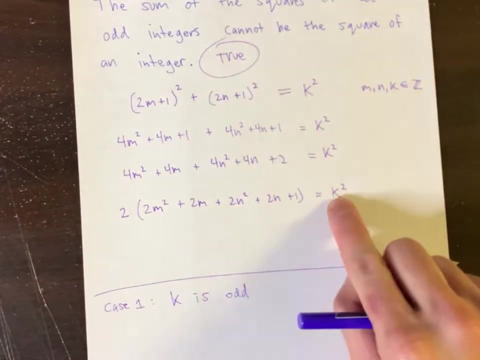 how about? let me take out a 2 from here? Here's what I want you to see: 2 times blah, blah, blah equals k squared. You know what that means? That means that 2 can divide k squared. Here are two cases. k is a number, It is an integer, It has two possibilities. 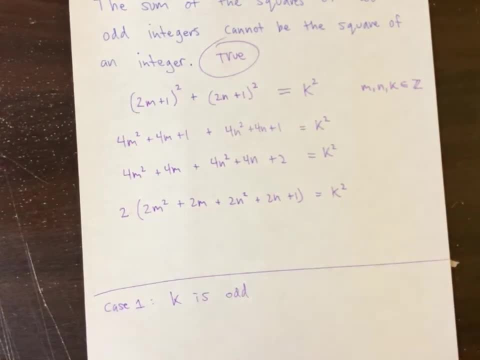 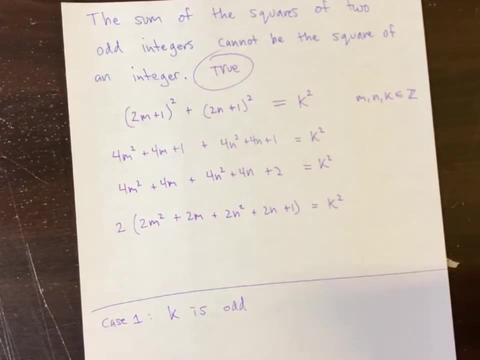 k can be odd or it cannot be odd, making it even. Those are the only two options. I can tell you k cannot be odd Because think about it like this: Let's pretend let me just make this up and then I'll scratch this off the paper. Let's pretend that k is 5.. If you plug in 5 for k, here it's. 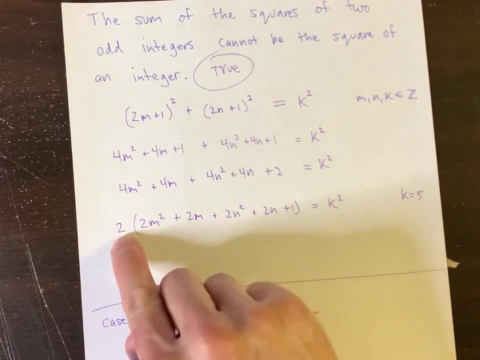 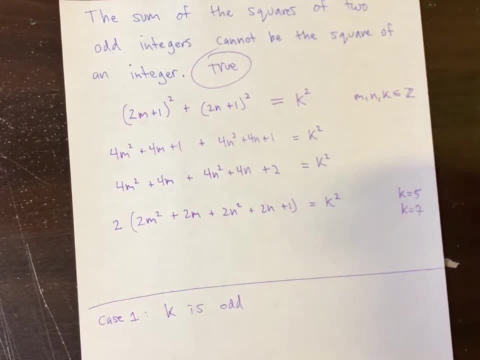 going to be 25.. Can 25 be divided by 2? No, 2 cannot go evenly into 25.. What if k is like 7? You know, 7 squared is 49.. Can 2 divide into 49? No, Because 2 can't go into. 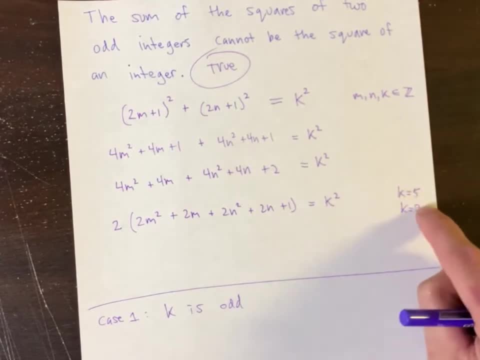 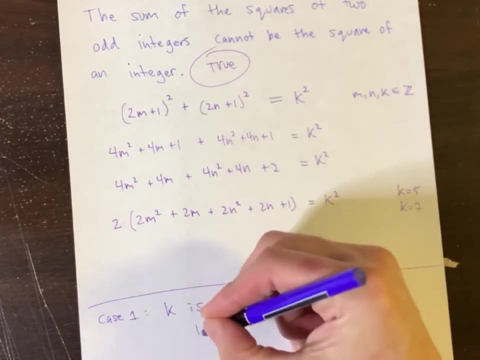 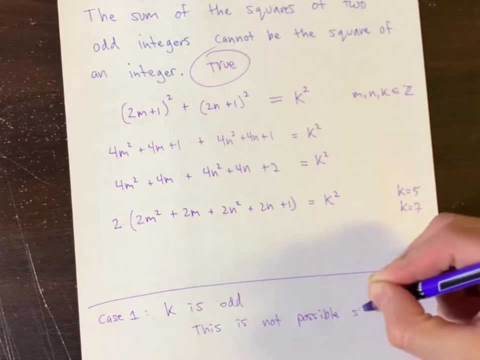 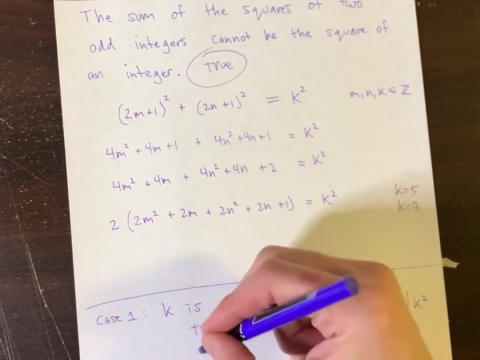 either of these numbers, much less the square of these numbers. So for that reason you can tell them this. So where k is odd the case when k is odd, you can say this: this is not possible. This is not possible, since 2 divides k squared. That implies that implies that 2. 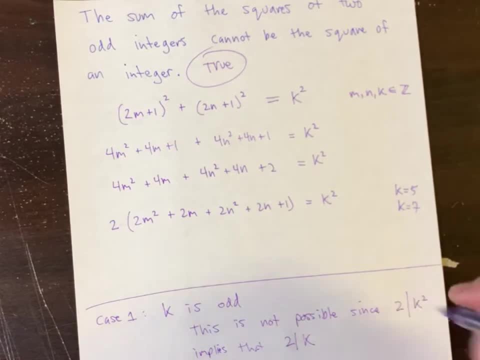 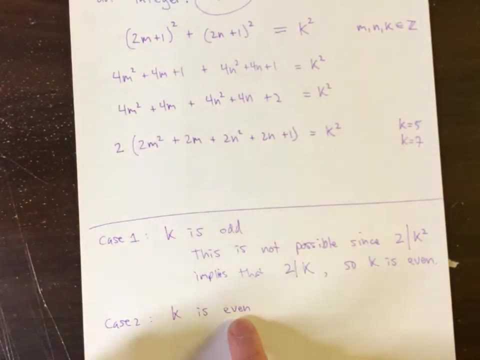 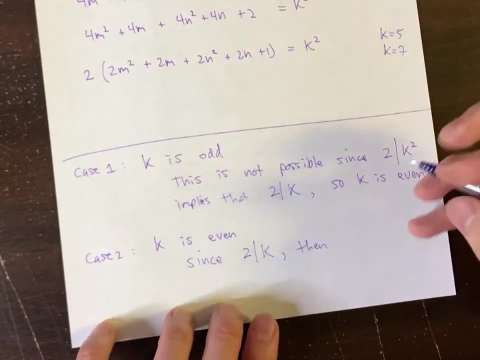 divides k, And if 2 divides k, then k is even. The only possibility now is that k is even, But I want to show you that even that is not possible Now, since 2 divides k comma, then that means that 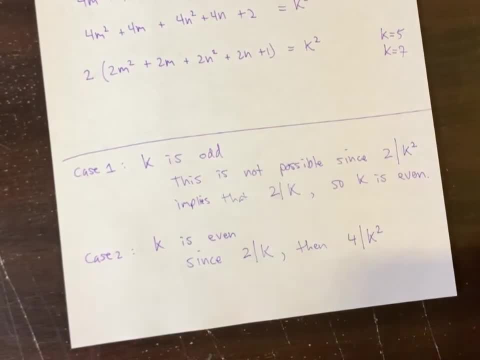 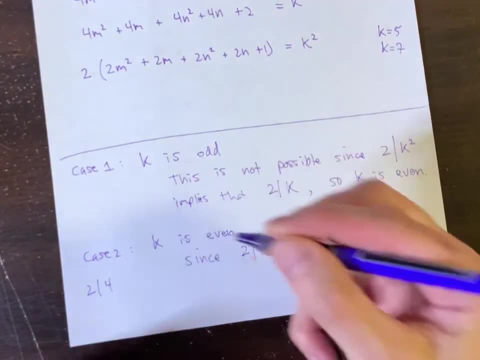 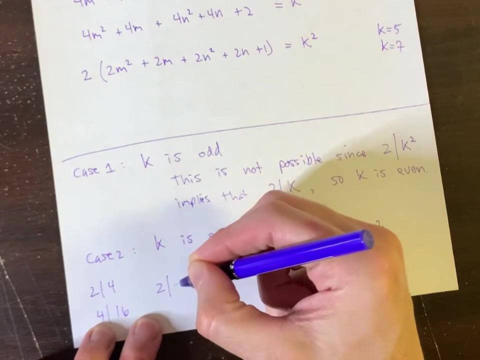 4 should divide the square of k, And that's what that means Like. for instance, if 2 divides k, think of an even number- 2 divides like 4.. If I square 2, that means 4 divides the square of that which is 16.. Here's another example: 2 divides. let's say: 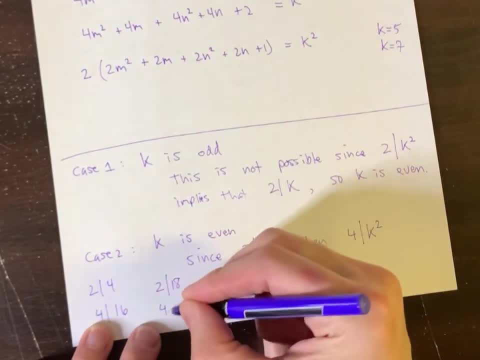 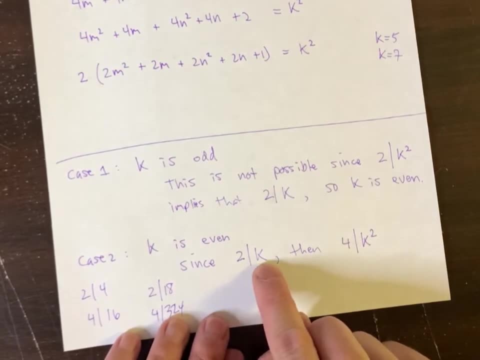 18.. And that means that the square of 2,, which is 4, is going to divide the square of 18,, which is 324, and so on and so forth. That's true. So if 2 divides a number, then the square of 2.